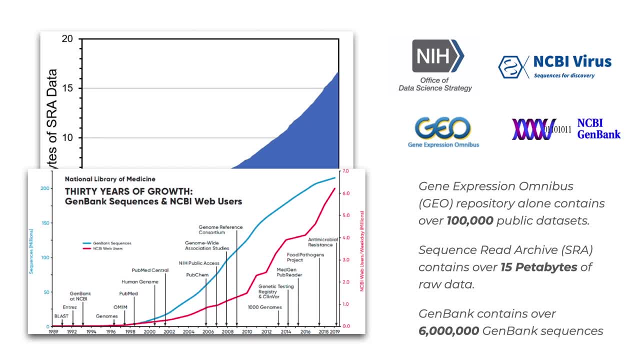 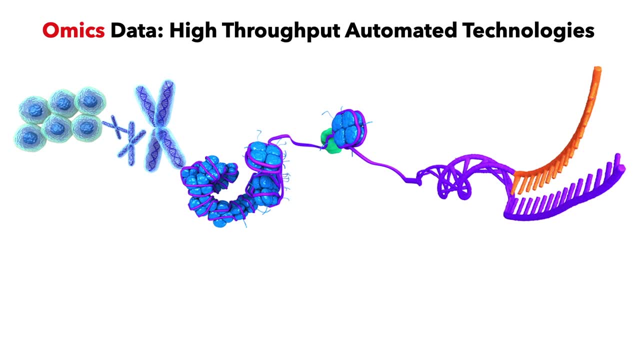 an exponential growth of gene bank sequences representing over 5 million different organisms. Not only is this a lot of data, but it's also data that is highly variable. There are many different formats and platforms for data generation, making it extremely heterogeneous. One key technology: 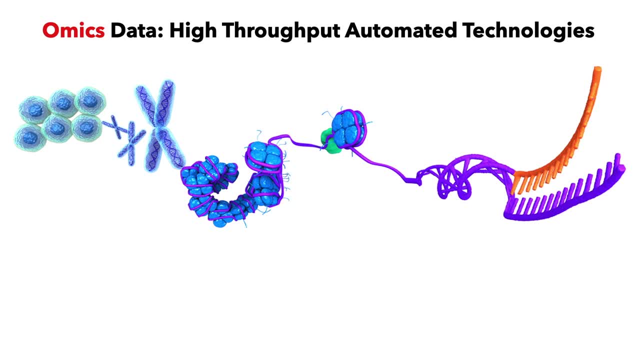 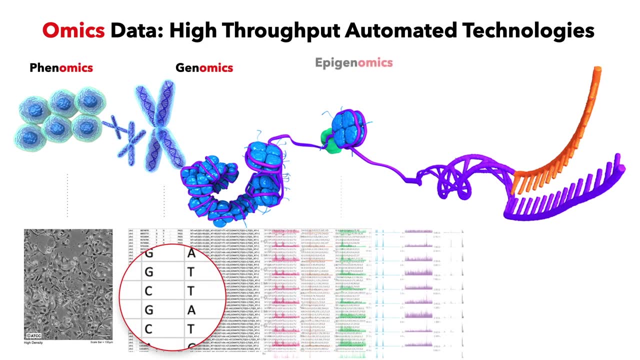 driving this explosion in data is omics. Omics technologies, like next generation sequencing, can be used to explore the roles, relationships and actions of the various types of molecules that make up the cell of an organism. Many types of omics data can be generated using next generation. 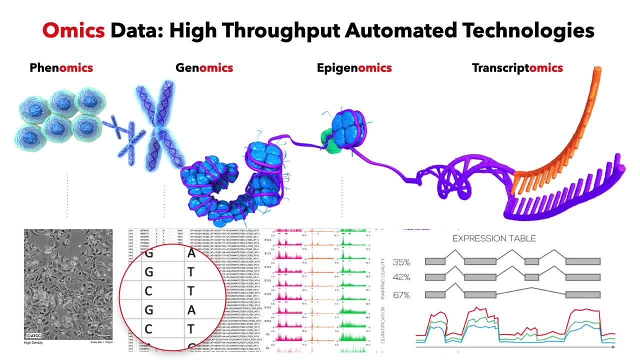 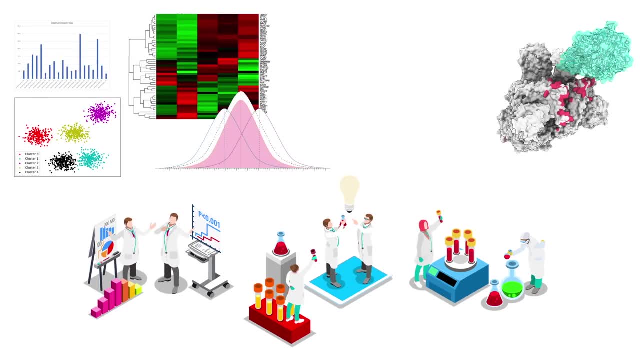 sequencing, or what is also known as high throughput sequencing. To analyze such data, novel computational technologies have been developed that are transforming life sciences, enabling biotechnology and empowering biomedical research. As a result, researchers are making new discoveries every day, Understanding this data, the technologies used to produce it, and taking 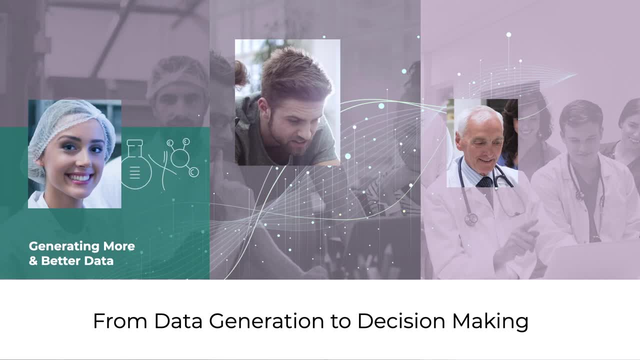 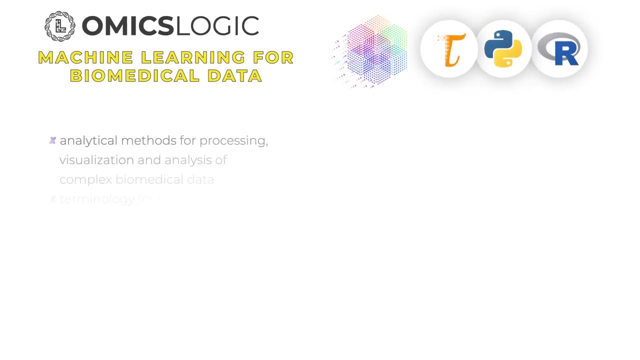 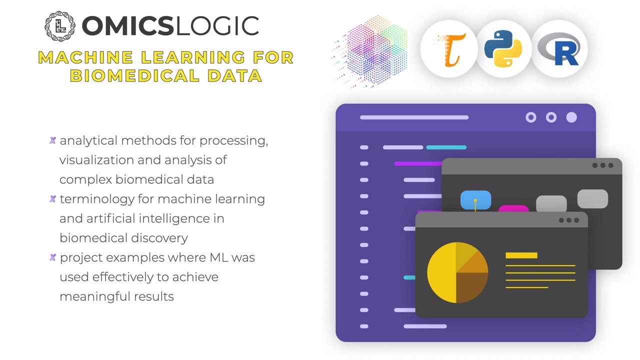 techniques for its analysis are now critical to understand for anyone across the whole life cycle of data, from lab technicians to data scientists and decision makers. In this program, you will learn about analytical methods for processing, visualization and analysis of complex biomedical data. You will understand the terminology for machine learning and artificial intelligence, and 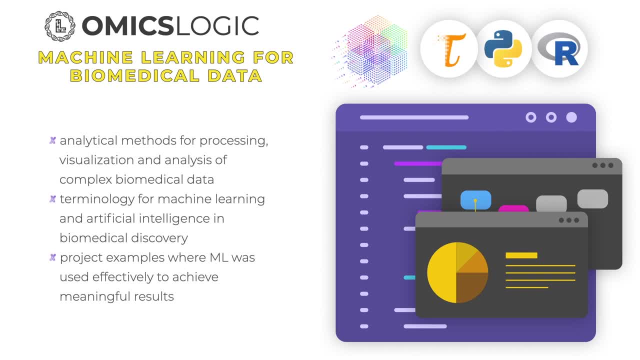 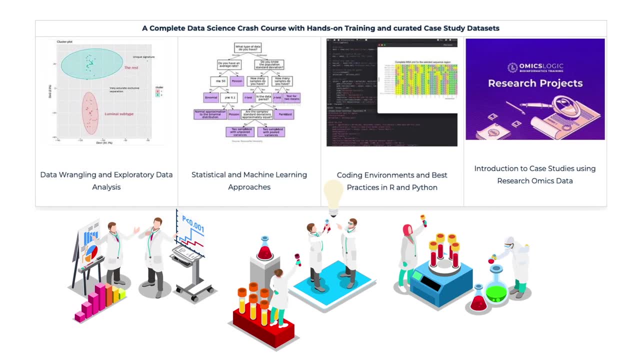 biomedical discovery and see project examples where machine learning was used effectively to achieve meaningful results. You will also hear about commonly used machine learning algorithms for analyzing omics data. understand the differences between machine learning models and problems. they can be applied to see the different applications of machine learning for omics studies and project. 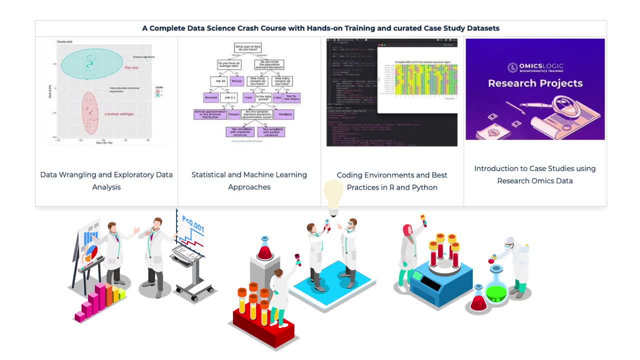 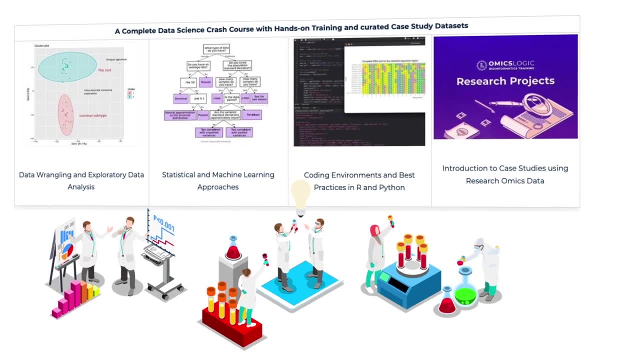 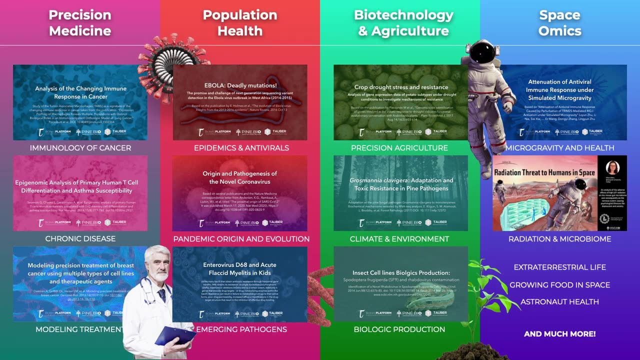 design objectives and gain experience with popular Python and R packages for data visualization, analysis and machine learning. Most importantly, you will learn to use your understanding to work on industrial and research problems of the 21st century – precision medicine, population health, biotechnology, agriculture and space omics. Each session is 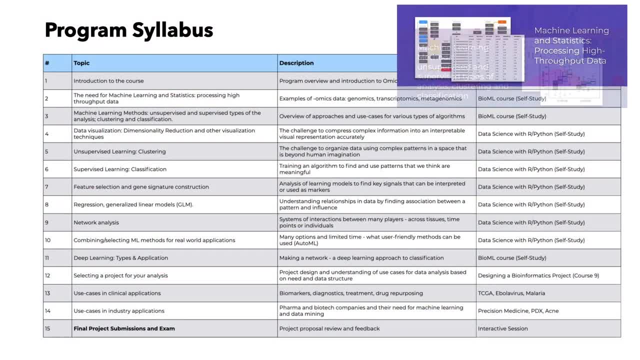 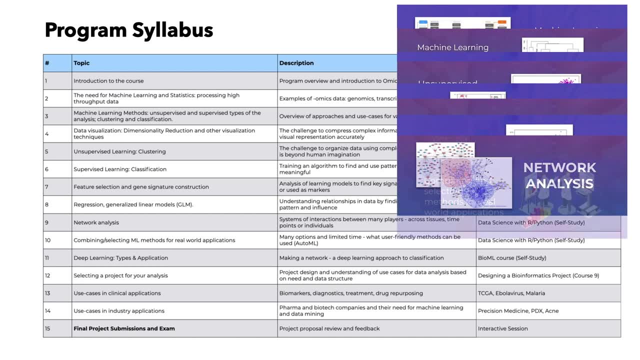 designed to cover the topics in a practical and informative way, starting from the very basics and covering topics appropriate for both intermediate and advanced levels. Depending on how far you want to go with this program, you can choose to stay within the scope of the syllabus.